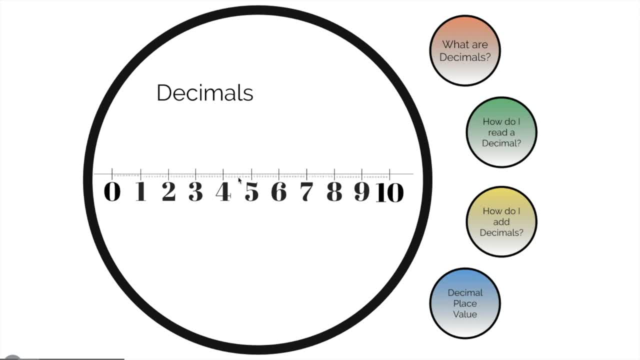 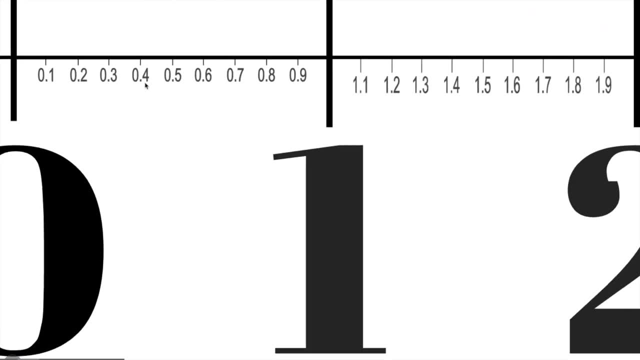 Anyways, we got our number line here, 0 to 10, and I'm gonna zoom in a little bit so that we can see where decimals are and notice that decimals are in between the numbers right, so between zero and one there are decimals. this decimal is, has a. 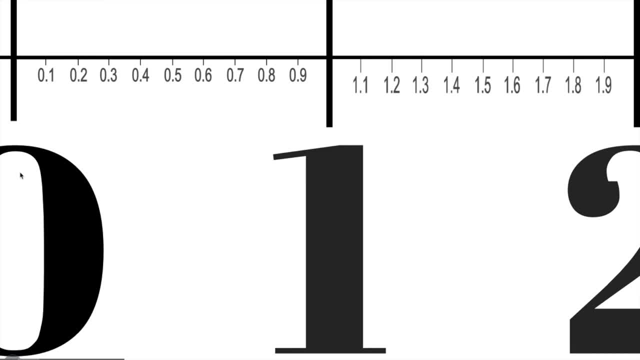 1 in the tens place, that's 1 tenth. it's less than 1, but more than 0.. One tenth, two 10ths, 3 10ths, 4 tenths, 5 tenths, 6 tenths, 7 tenths, 8 tenths, 9 tenths and. 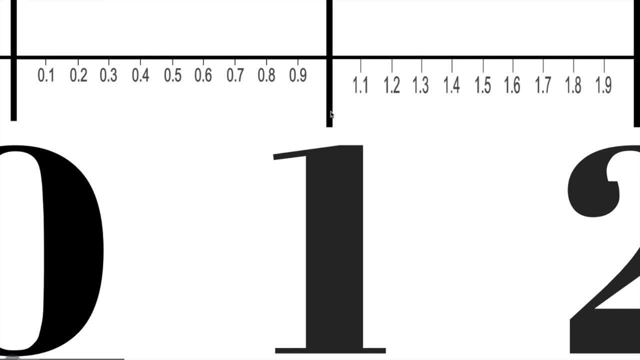 then 10 tenths would be one whole right. and then this right. here this decimal is more than one, but less than 2. this is 1 and 1 tenth. this is 1 and 5 tenths- unbelievable one and nine tenths. again all of these decimals here, more than one, but less than two. now let's. 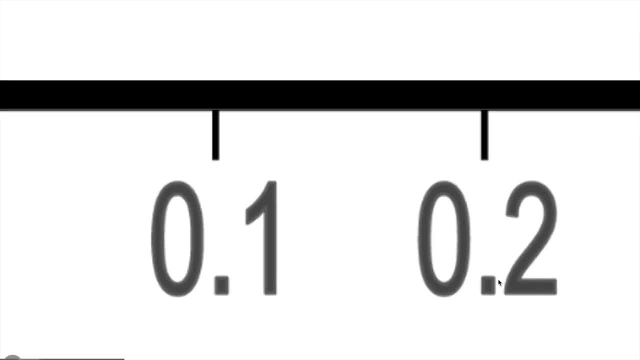 zoom in even closer. all right, so in between the tenths would be hundredths. oh, all right. so for example, this has a five in the hundreds place, that's five hundredths less than one tenth, but still again more than zero. eight hundredths, okay, nine hundredths, and then 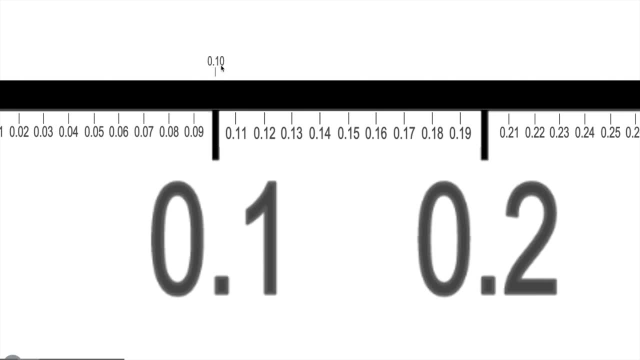 right here where one tenth is. that's the same thing as ten hundreds. ten hundredths and one tenth are equivalent to each other, and you've probably seen the last video already, where you can see that one tenth and ten hundreds are exactly the same. uh, fifteen hundreds more than. 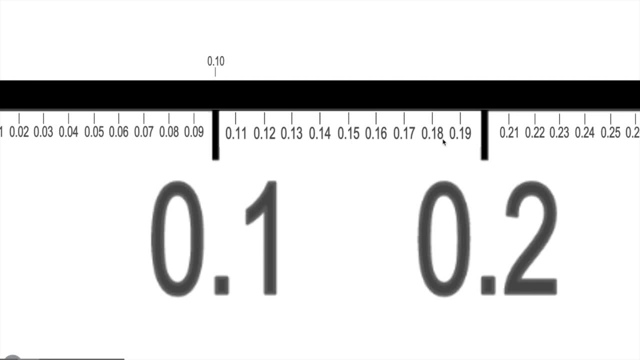 one tenth, but less than two tenths. seventeen hundreds, eighteen hundreds, nineteen hundreds and then twenty hundreds would be right here where two tenths is? you notice both of them have a two in the tenths place. they are equivalent. okay, and then twenty one hundred, twenty two hundred, twenty three hundreds, again more than. 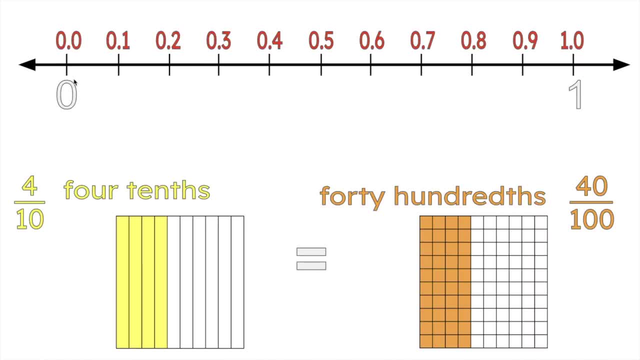 two, but less than three. resuming in here: zero to one. well, i broke it into ten equal parts: one, two, three, four, five, six, seven, eight, nine, ten equal parts, and so now it's easy to find where my tenths are going to go. so if this is four tenths, well, this is four. in the tenths place, you would read: